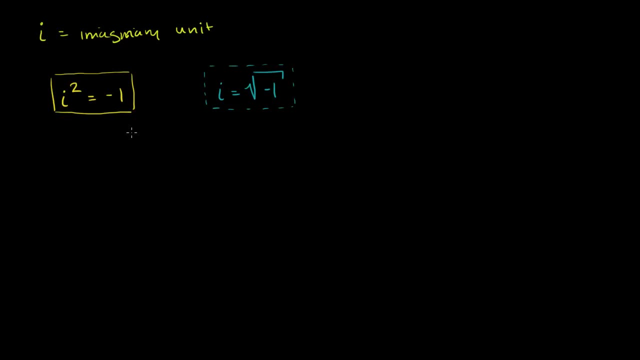 we'll learn in the future complex numbers, But for your understanding, right now you don't have to differentiate them. You don't have to split hairs between any of these definitions. Now, with this definition, let's just think about what the different powers of i are. 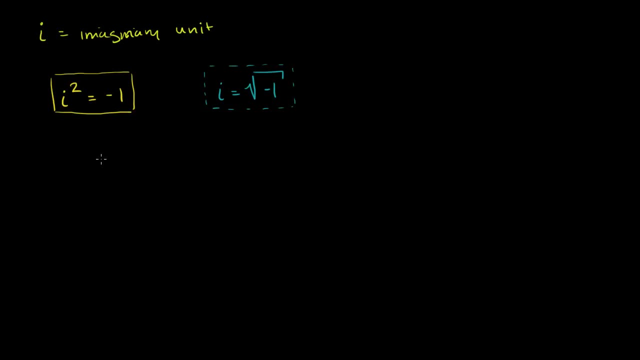 Because you can imagine if something squared is negative 1, if I take it to all sorts of powers, maybe that should give us all sorts of weird things, And what we'll see is that the powers of i are kind of neat because they kind of cycle, or they do cycle through a set. 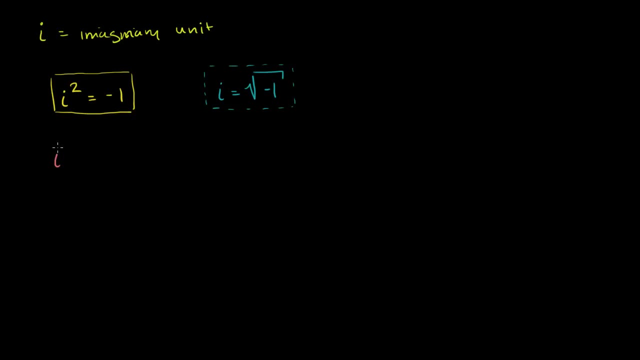 of values. So I could start with i to the 0th power, And so you might say: hey look, anything to the 0th power is 1.. So i to the 0th power is 1, and that is true. 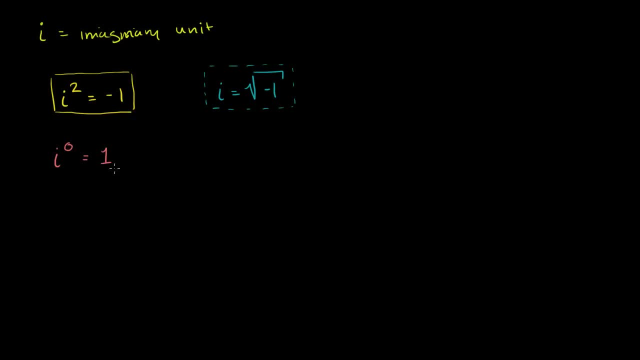 And you could actually derive that even from this definition. But this is pretty straightforward: Anything to the 0th power, including i, is 1.. Then you say, OK, what is i to the first power? Well, anything to the first power is just that number. 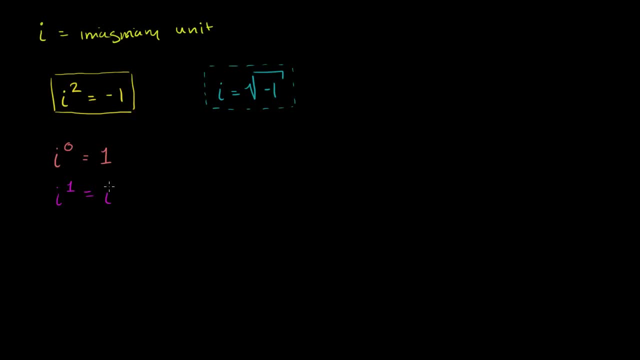 times itself once. So that's just going to be i, really, by the definition of what it means to take an exponent, So that completely makes sense. And then you have i to the second power. Well, by definition, i to the second power is equal to. 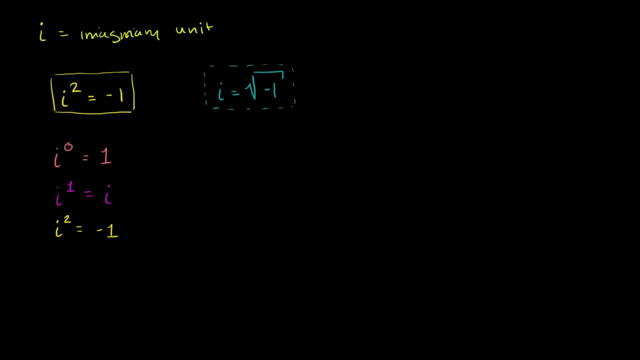 negative 1.. Let's try: i to the third power. I'll do this in a color I haven't used. i to the third power. Well, that's going to be i to the second power. times i, And we know that i to the second power is negative 1.. 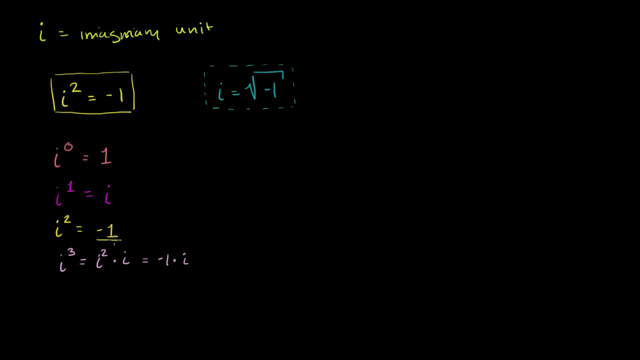 So it's negative 1 times. i Let me make it clear: This is the same thing as this, which is the same thing as that i squared, is negative 1.. So when you multiply it out, negative 1 times, i we'll. 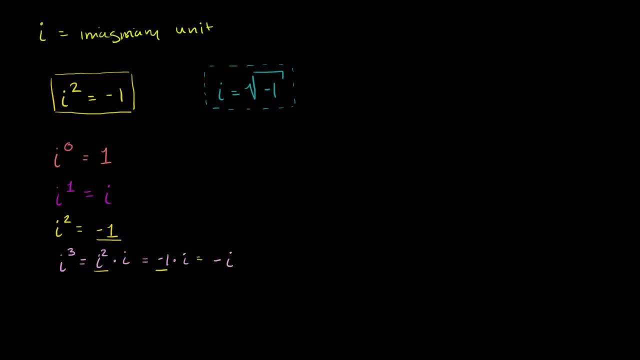 write as negative i. Now what happens if we take i to the fourth power? I'll do it up here: i to the fourth power. Well, once again, this is going to be i times i to the third power. So that's i times i to the third power. 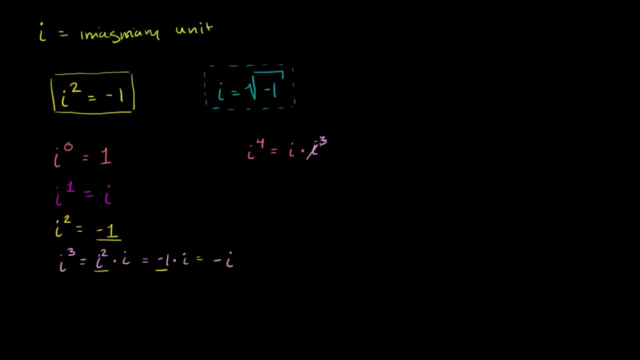 But what was i to the third power? i to the third power was negative i. This over here is negative i, And so i times i would give you negative 1.. But you have a negative out here, So it's i times i is negative 1.. 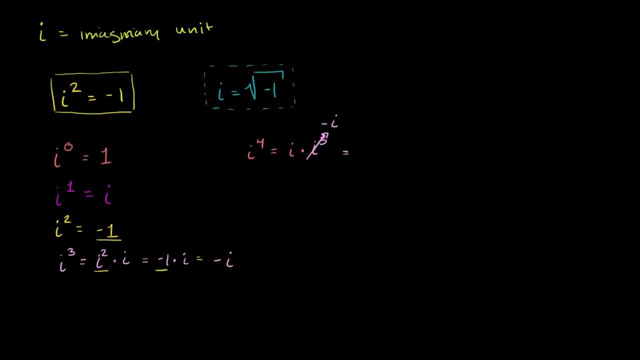 And then you have a negative That gives you positive 1.. Let me write it down. So this is: i times negative i, which is the same thing as negative, 1 times. remember, multiplication is commutative. If we're just multiplying a bunch of numbers, we can. 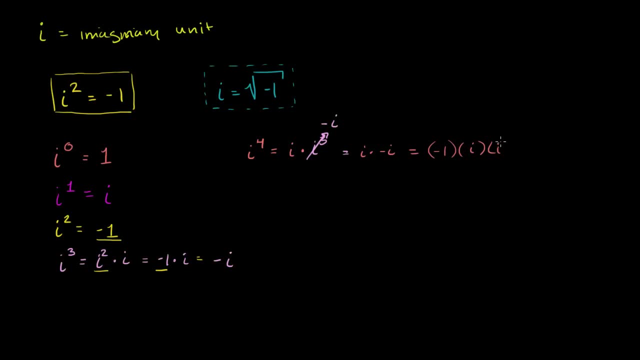 switch the order. This is the same thing as negative 1 times i times i. i times i by definition is negative 1.. Negative 1 times negative 1 is e Negative. 1 times negative 1 is e Negative. 1 times negative 1 is equal to 1.. 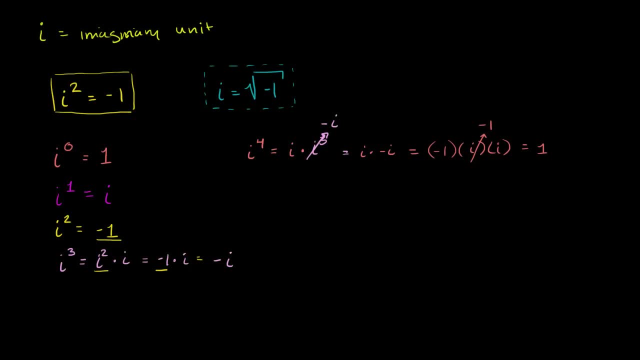 So i to the fourth is the same thing as i to the zeroth power. Now let's try i to the fifth power. Well, that's just going to be i to the fourth times i, And we know what i to the fourth is. 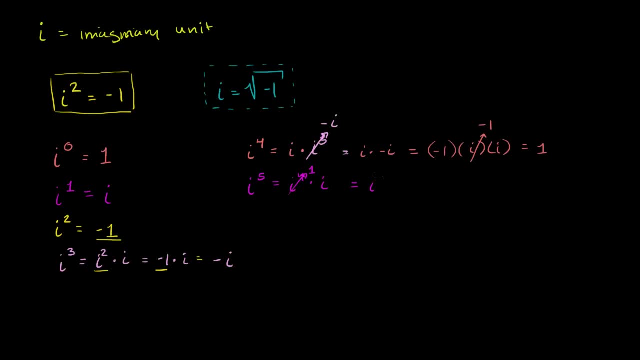 It is 1.. So it's 1 times i, or it is just i again, And so once again, it is exactly the same thing as i to the first power. Let's try, and just to see the pattern keep going, let's try. 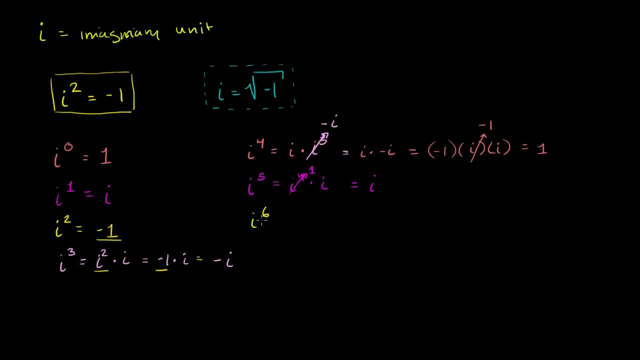 i to the sixth power. i to the sixth power. Well, that's i times i to the fifth power. That's i times i to the fifth. i to the fifth, we already established is just i. So it's i times i. 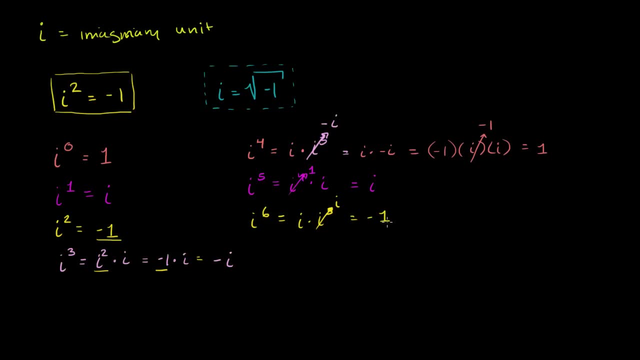 It is equal to: by definition, i times i is negative 1.. And then let's finish up. Well, we could keep going on this way. We can keep putting higher and higher powers of i here, And we'll see that it keeps cycling back. 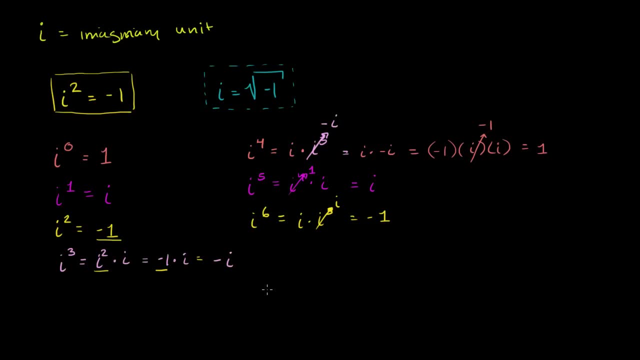 And in the next video I'll teach you how taking an arbitrarily high power of i, how you can figure out what that's going to be. But let's just verify. this cycle keeps going. i to the seventh power is equal to i times i to the sixth power. 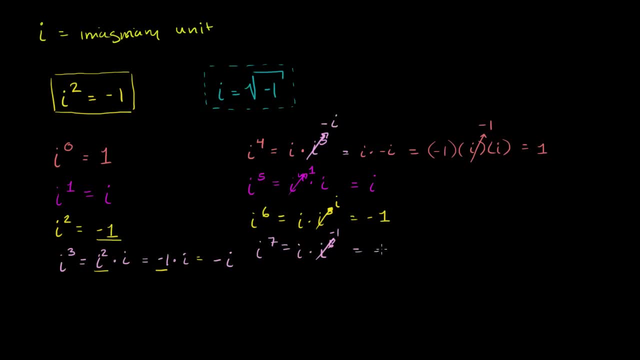 i to the sixth, power is negative 1.. i times negative 1 is negative i, And if you take i to the eighth once again, it'll be 1.. i to the ninth will be i again. so on and so forth.